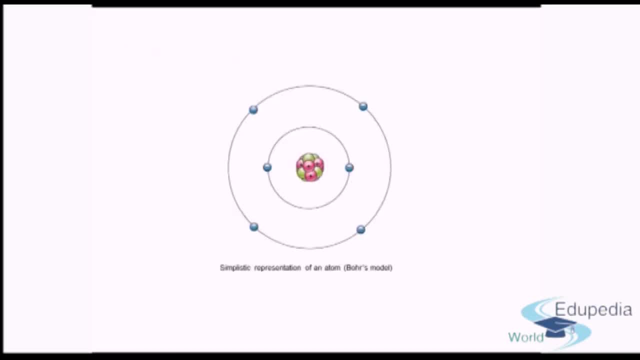 This necessitates the understanding of atomic structure. To begin with, let us see the very basic structure of a simple atom. This is the simplistic representation of an atom as presented by Bohr. in Bohr's model, As we can see, here are some particles with a negative charge. 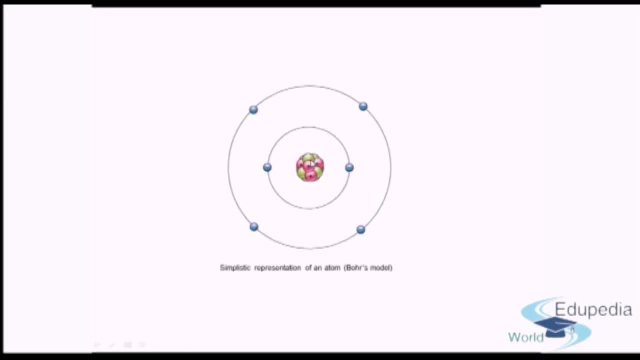 Here are some particles with a positive charge, and the green particles are supposedly chargeless. Let us see each of them individually, one by one. The negatively charged particles which seem to move in orbits around a center, is known as electron, So electrons are basically negatively charged particles. 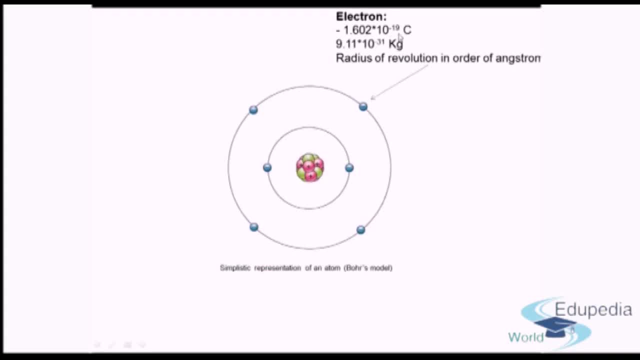 What are the properties of an electron? Electron is having a charge of minus 1.602 into 10 to the power minus 19 coulomb. Okay, that is the charge. What is the mass of electron? It is 9.11 into 10 to the power minus 31 kg. 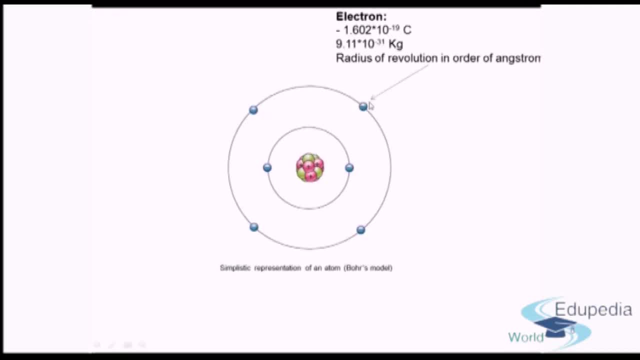 It is in the order of minus 32 kg. And finally, as I said, this electron seems to revolve around a center. This electron seems to revolve around a center. This electron seems to revolve around what is known as nucleus. This is the nucleus of the atom and the radius of revolution. that is the distance from here. 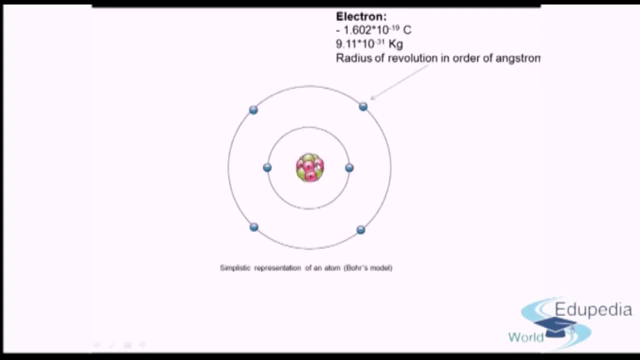 The center to this place is in the order of angstrom, And that is what defines the atomic size. The distance from the center to the outermost electron Roughly gives you an idea about the atomic size. Next let's see what are these positive particles. These positive particles are known as protons. 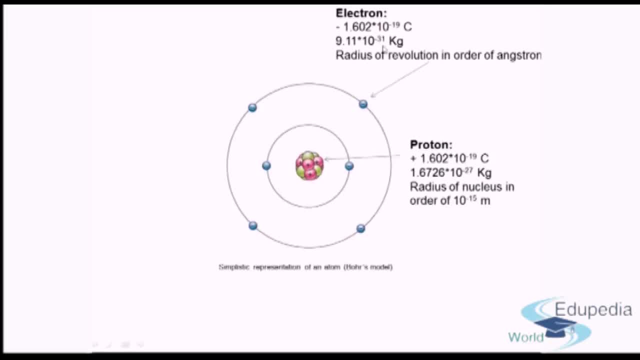 and similar to the charge of the electron, which was negative: 1.602 into 10 power minus 19 protons have same magnitude but are oppositely charged, that is, they are positively charged and have same magnitude. The point of difference is the mass. The mass of electron was in the order. 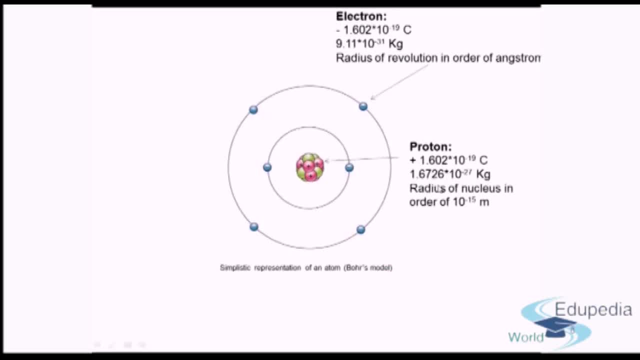 of 10 to the power minus 31, whereas the mass of proton is in the order of 10 to the power minus 27. that is four orders of magnitude different. So a proton is much more heavier than an electron. Then third part is, as I mentioned, the central region which homes the proton is known as the 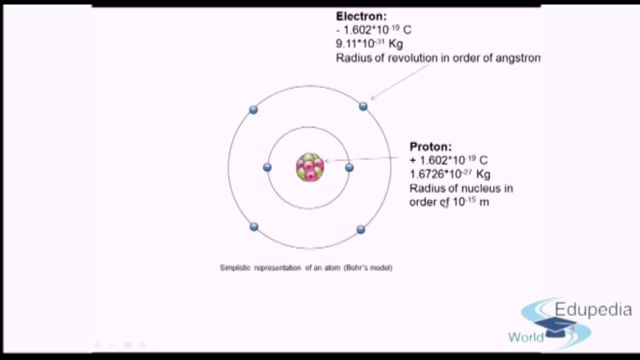 nucleus of the atom. and the nucleus of the atom is in the order of 10 to the power minus 15 meters. So the radius of the nucleus is kind of 10 to the power minus 15 meter, which is a distinctive point of difference from the radius at which the electrons revolve around the nucleus, which was 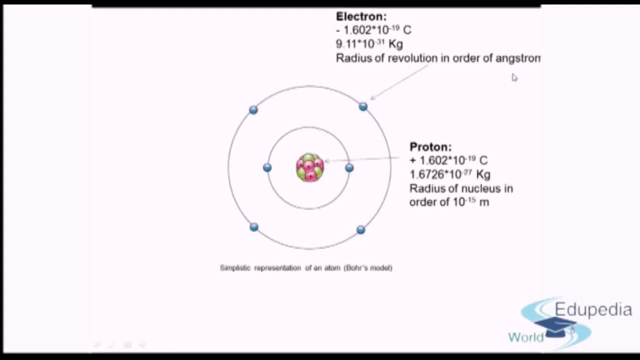 angstrom, that is 10 to the power minus 10 meter. Now let us see the third kind of particle that constitute the atom: the green particles. The green particles are known as neutron. What is a neutron? Neutron is a charge less particle, that is, it has zero charge. The mass is very similar to 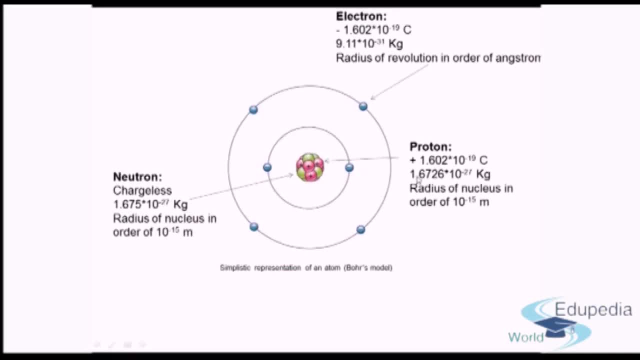 that of a proton. It's very, very slightly more than that of a proton. It is 1.675 into 10 to the power minus 27 kg, and thereby even a neutron is kind of four orders of magnitude heavier than an electron and the same radius, that is the radius of nucleus, in the order of 10 to the power minus 15 meter. 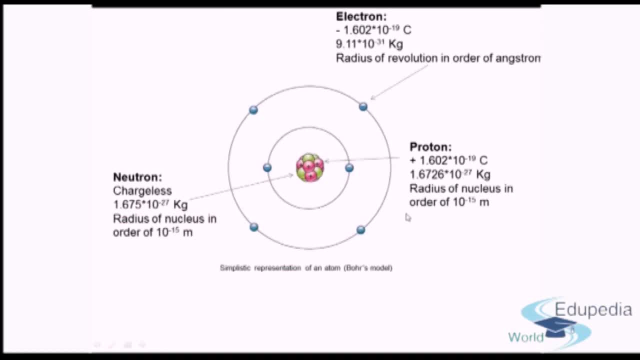 As that of the proton. Now, the interesting take home from here is, if you observe, the heavy particles, that is, the proton and the neutron, both reside in the nucleus, Isn't it? The very light particles, electron, revolve in these orbits. Therefore, the mass of the atom almost completely resides at the 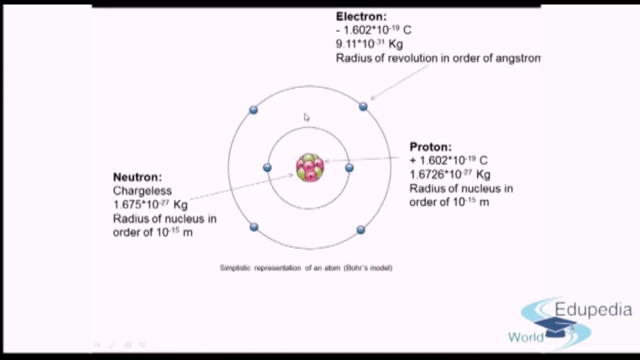 center or resides at the nucleus of the atom. Now the proton and the neutron are the same. The neutron together is what is called as the nucleus. So this is my nucleus. and in a particular atom, if the atom is supposed to be electrically neutral- and how is that possible? That is possible. 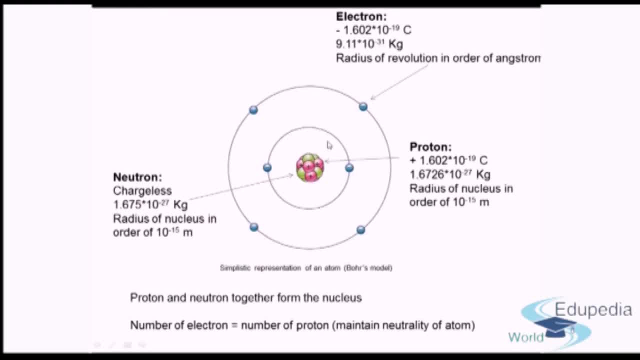 only when the number of electrons and the number of protons are same. Thereby, the negative charge imparted by all the electrons will be counteracted by the positive charge imparted by all the protons. In order to maintain the neutrality of an atom, the number of electrons is equal to the number of protons. 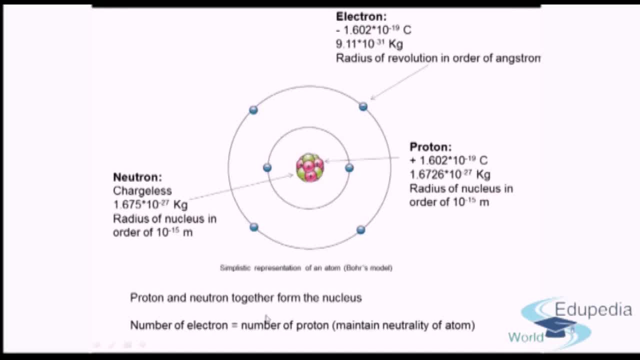 This whole description is the basic Bohr's model description in which the electron revolves around the nucleus in fixed orbits. We'll see this in details in the next slide. Now let us familiarize ourselves with a few terminologies. Atomic number: The atomic number represented by a capital Z. 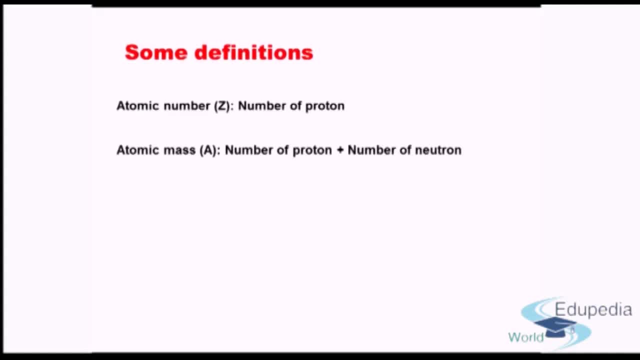 represents the number of protons. Atomic mass is the sum of the number of proton and the number of neutron. As I said, the bulk of the mass lies in the nucleus, that is, within the proton and the neutron. Therefore, the electrons are not going to come into the picture. Then a mole is defined as: 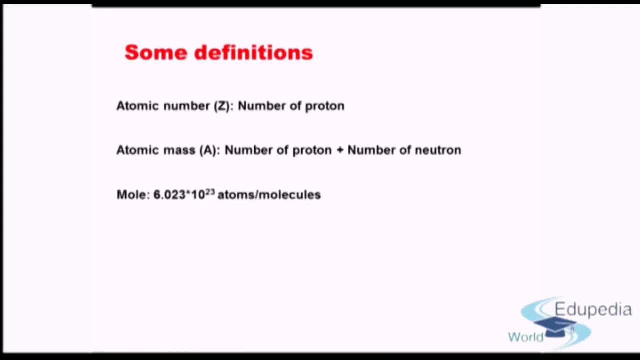 six point zero, two, three into ten, to the power twenty three. atoms or molecules. That is the definition of a mole. An isotope is rather two. materials which has same atomic number but different mass number are known as an isotope. To give you an example, an isotope would be chlorine. 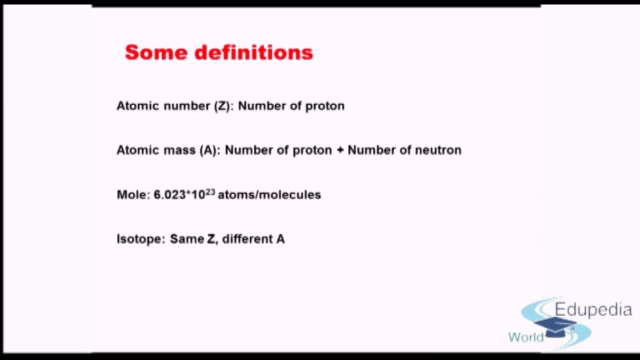 thirty five and chlorine thirty seven. Both have atomic number seventeen, but chlorine thirty five has a mass number thirty five, whereas chlorine thirty seven has a mass number thirty seven. Isotopes: OK, So this gives you a brief definition of the different terminologies. 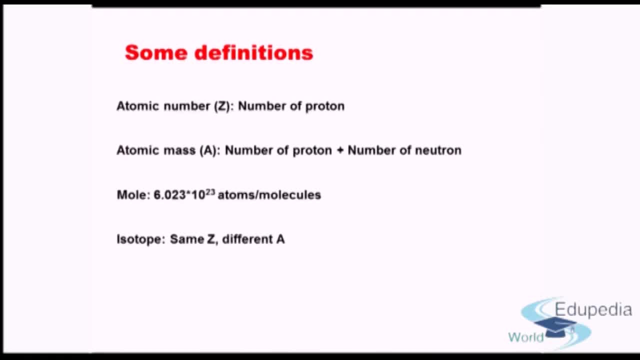 pertinent with atomic structure. Next we'll see the Bohr's model in description. We'll see what is the limitation of Bohr's model and how that gives rise to what is known as wave mechanical model. and what does that mean? OK, So this is the same picture which we saw while discussing. 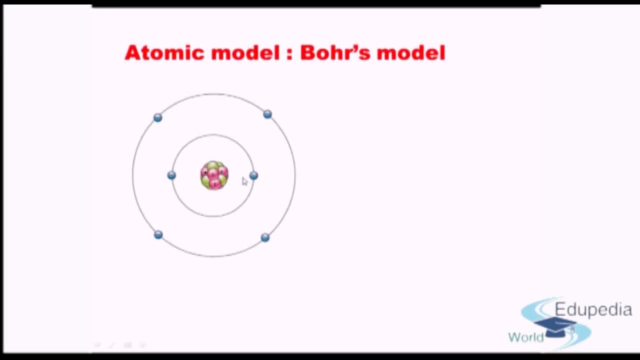 the atomic structure. This was the simplistic picture known as the Bohr's model. In the Bohr's model, the electrons revolve around the nucleus in fixed orbits. So these are the orbits in which the electron revolve around the nucleus. They cannot revolve in any arbitrary orbit, That is. 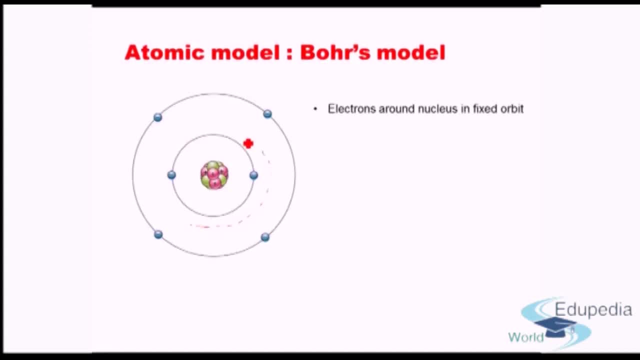 to say you cannot have an orbit intermediate between two defined orbits, and electron will not revolve around the nucleus. This is the initial definition. So the energy of electron is quantized. So the energy of electron is quantized. This is the end to end definition of Bohr's model. 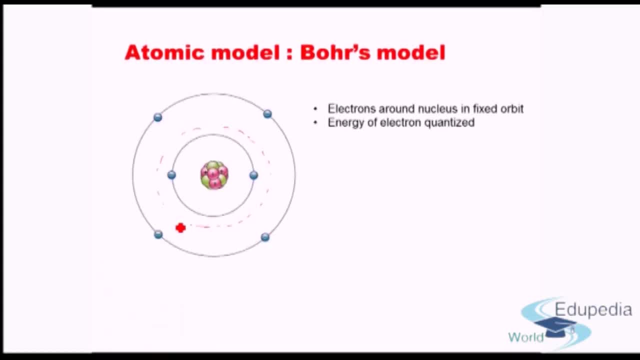 Now, since we have said that the electrons are revolving around in fixed orbits, The energy level will be defined by the orbit. Therefore, the energy is quantized. It cannot take up any value it wants. It has to be either the energy level at this Radius or the energy level at this radius. 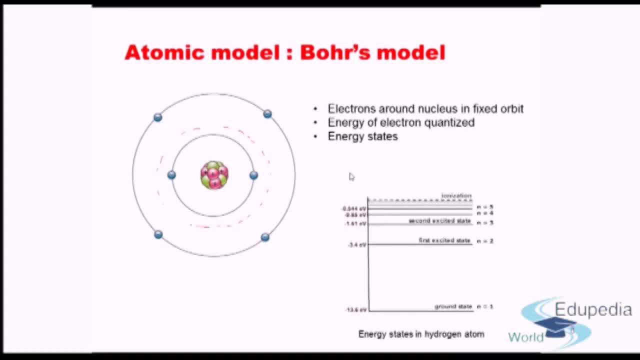 quantum radius. now, this quantization of the locations at which electrons can be present results in what is known as energy states. see over here what you can observe: there is a orbit which is closest to the nucleus in which the electrons can revolve. then there is a second. 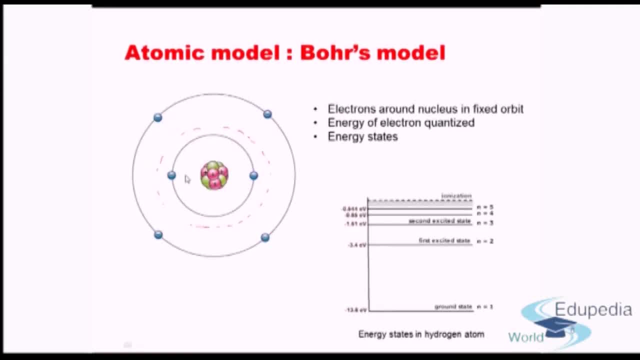 closest orbit. so there are states of orbit, and each state has a particular energy associated with it. therefore, what we can say is these are energy states in which the electron can revolve. the radius closest to the nucleus in which the electrons revolve is known as the ground state. 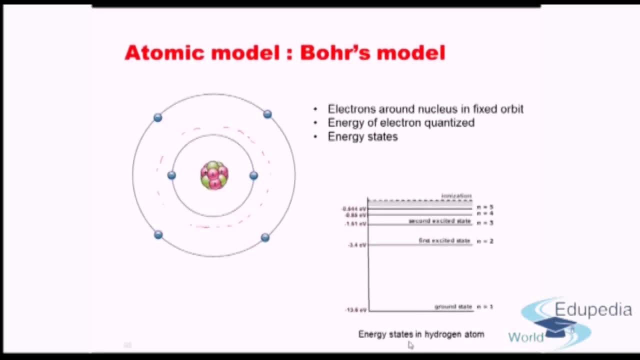 this is the energy representation for a hydrogen atom. drive home the point. we are using hydrogen atom, which is the simplest atom, because it has one electron. now the electron, ideally, will be at the lowest energy state, that is the orbit which is closest to the nucleus, and we define the energy at infinity. that is very. 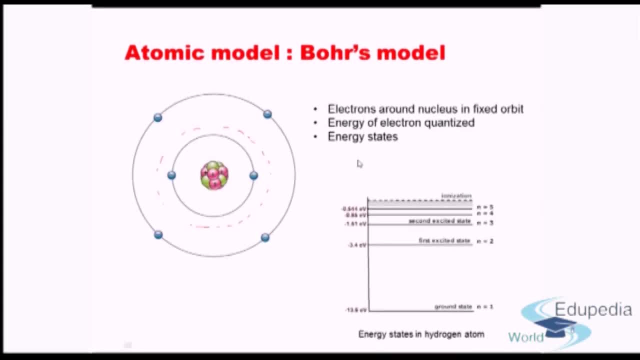 very far away from the nucleus, as zero electron volt. and then, after calculations, it is found that for the hydrogen atom at the lowest energy state the energy level for the ground state turns out to be minus 13.6 electron volt. but suppose we give some energy into the electron which is at the 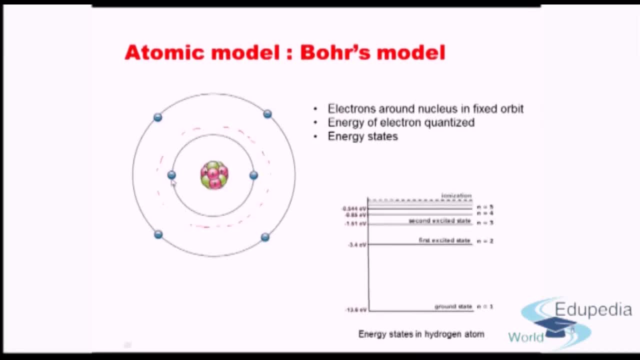 lowest energy state. what it will do? it will absorb that energy and jump to a higher state, such that it has sufficient energy to jump from the first state to the second state. then the energy will increase from minus 13.6 electron volt to minus 3.4 electron volt. similarly, we can increase the 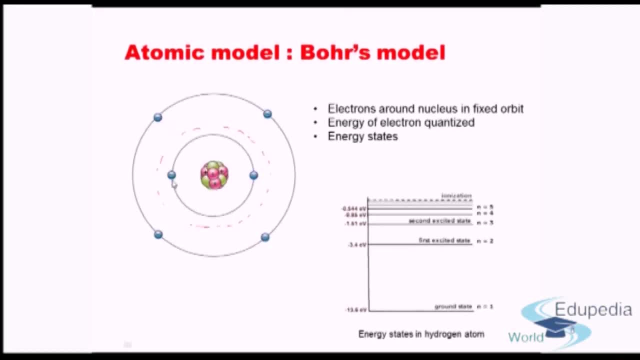 amount of energy input and we can keep pushing the electron further away from the nucleus and each of this state is a energy state. this lowest energy state is the ground state and the energy is the ground state. then the first excited state, second excited state and, if you give sufficiently high. 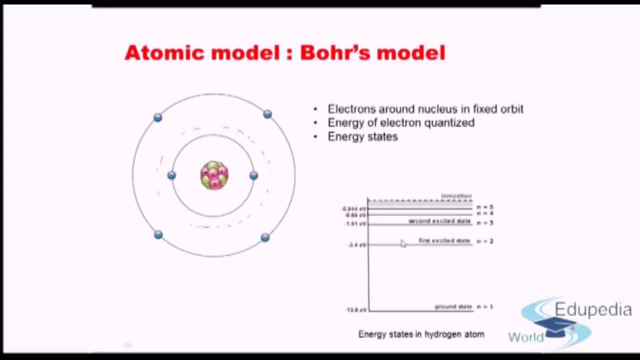 amount of energy, then what is known as ionization can take place. what happens in ionization? the electron is completely rejected from the atom. that is, electron gains sufficient amount of energy to be freed from the atom and the atom will develop a single positive charge because it has lost a 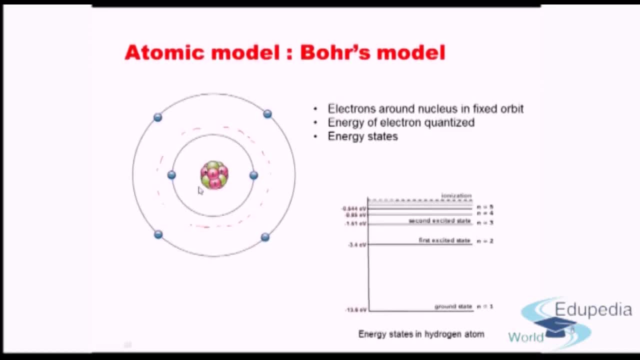 single negative charge. okay, so this was the basic idea behind the bohr's model. now, what is the drawback of bohr's model? bohr's model defines definitive orbits in which electrons can revolve, but what we know is that any charged particle which is accelerating will lose energy. this is the fundamental 101 of physics. 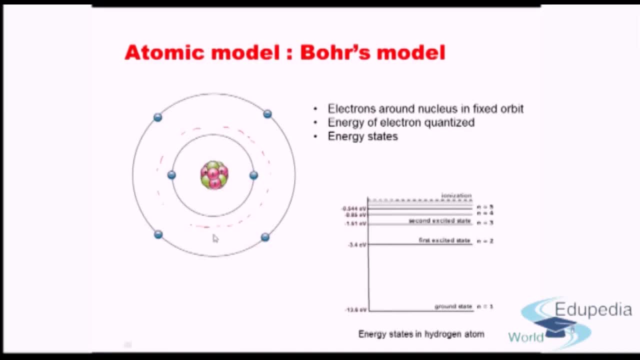 okay, therefore, these electrons which are revolving. revolution is accelerated motion. therefore, the electrons should not be able to revolve. they should not be able to revolve. they should not be able to keep moving in the same path. it should slowly lose energy and spiral down into the nucleus. 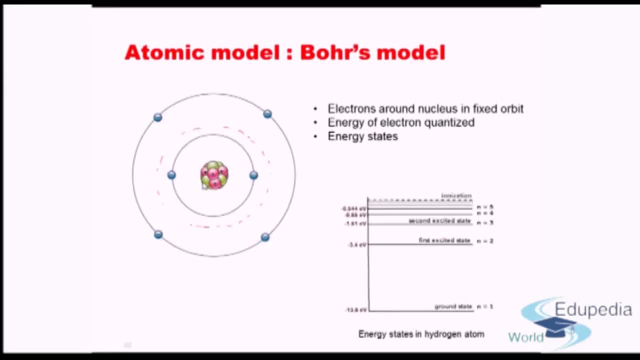 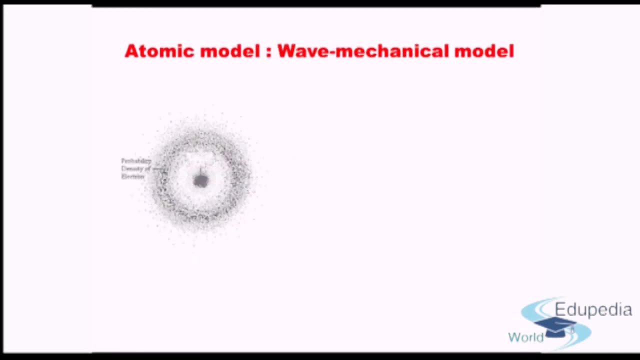 that does not happen thereby. there is some drawback, obviously in the bohr's model, which it does not account for. this led us to the development of what is known as wave mechanical model and wave mechanical model. let's see. what does it talk about? wave mechanical model, the 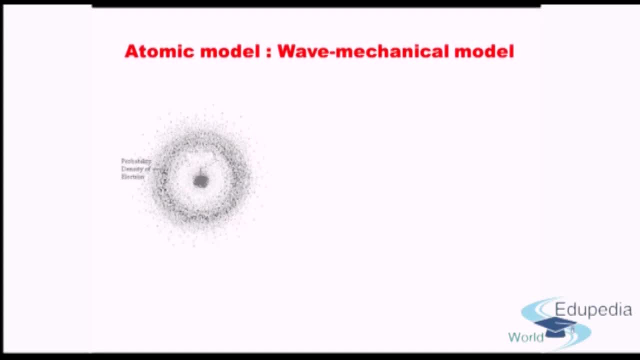 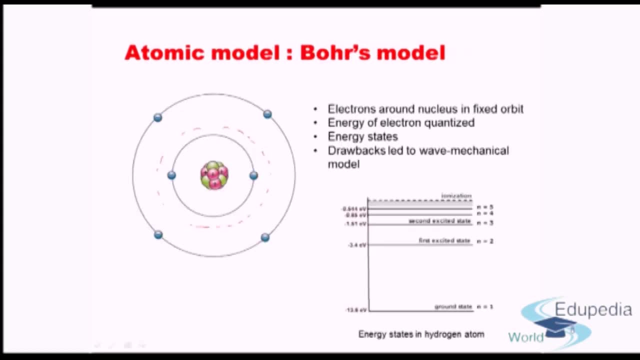 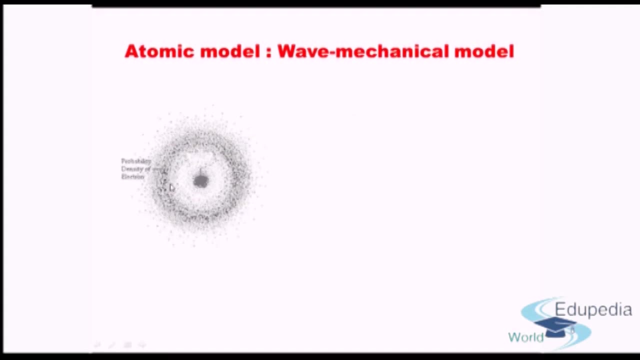 only difference between wave mechanical model. major difference between wave mechanical model and bohr's model is that bohr's model defines specific paths. right, you have a path here or here, whereas wave mechanical model says that electrons do not move in specific path. rather, you have probability distribution of regions where electron can be found. there will be some region where the 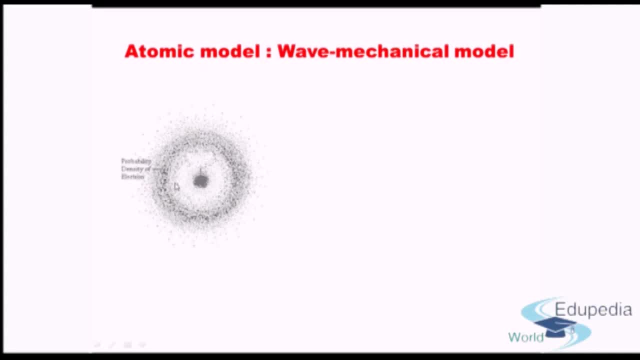 probability of finding electron is more. there will be some region. the chances of finding electron will be less. but you can't do it alone, cannot specify that this is the orbit. there will be a range of orbits with probability at different location. this leads to what is known as a electron cloud, because you're not specifying where exactly. 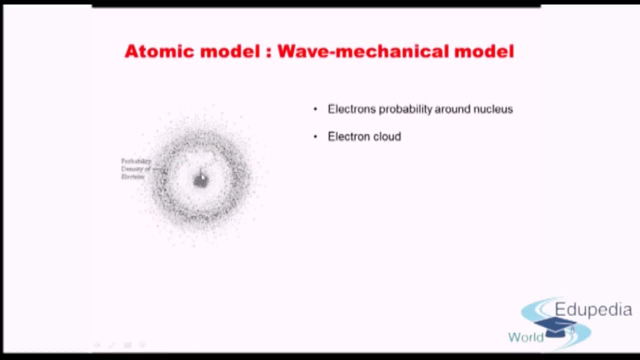 the electron is. it can be anywhere in this whole bound region. this is my nucleus and this wave mechanical model comes up from the idea that electron, like a wave, has a dual nature, that is, electron can sometimes behave as a wave and sometimes as a particle. now let me try to show. 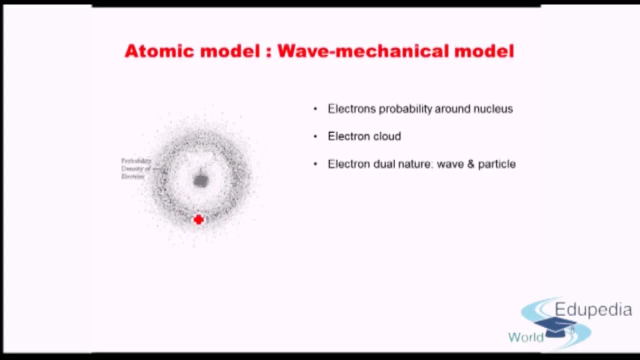 you how the probability distribution will look like. this is the electron cloud but, specifically speaking, suppose that this is my probability and this is my radius, okay. okay, this is a nucleus which is lying over here and i'm trying to draw the probability along this path. okay, so what is observed is very close to the nucleus. the probability of finding the electron 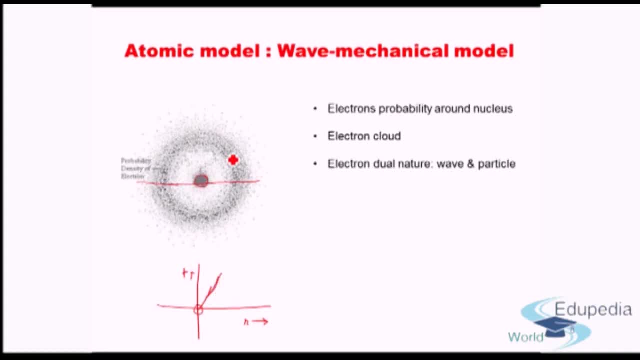 is almost zero. the probability keeps rising, rising and near the force orbit radius the probability is maximum and after that it starts to decrease again and it tends to zero at infinity. okay, so there is a probability to find electrons even at a very, very far distance, but the probability is 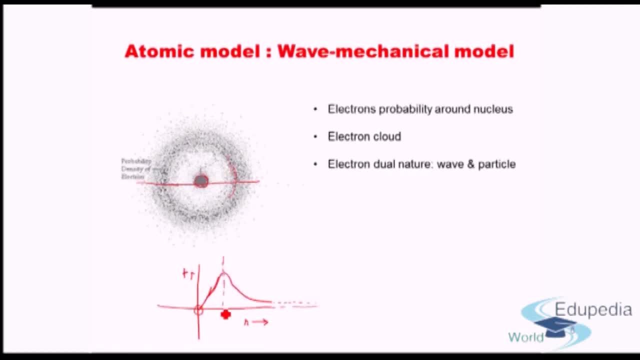 very less. the probability to find electron is maximum at bohr's radius, but it's not 100 percent. at bohr's radius there's a clear distribution and this kind of solves the problem which we encountered in the bohr's model, whereby accelerated electrons should lose energy and spiral down into the nucleus. 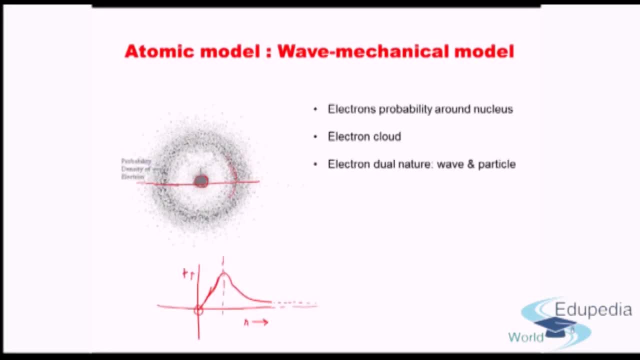 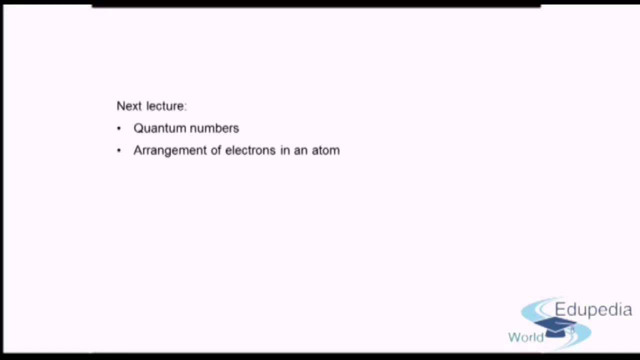 okay, so this brings us to the end of the lecture on the basic structure of a atom. we discussed bohr's model. we discussed the components of a nucleus. we discussed the wave mechanical model and how it is better than the bohr's model. next lecture, we'll focus on what are known.